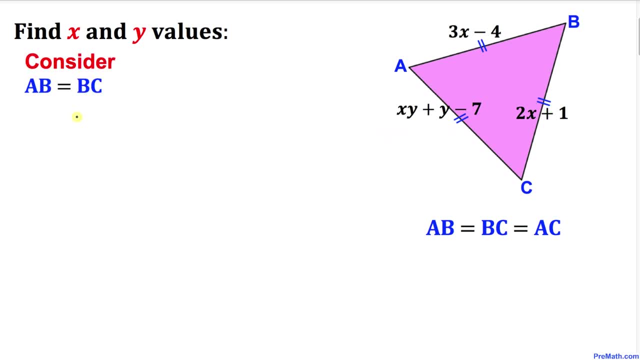 go ahead and get started with the solution, and here's our very first step. let's consider this side length a b equal to side length b c, and we know our side length a b is 3 x minus 4, and this, our other side length b c, is 2 x plus 1, so we can write this one as 3 x minus 4. 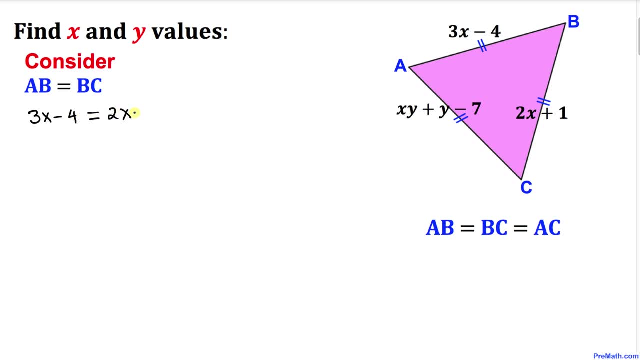 equal to 2 x plus 1. now let's move this: 2 x on the left hand side and negative 4 on the right hand side, so we are going to get 3 x and then minus 2 x equal to 1 plus 4, so thus 3 x minus. 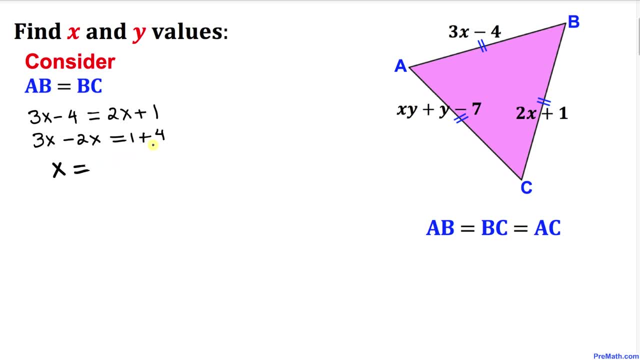 2 x is going to give us x equal to 1 plus 4 is 5, so our x value turns out to be 5, and here's our next step. let's consider this side length a c equal to side length b c. in our case, our side length a c is x y plus y minus 7, and our side length b c is 2 x plus 1. 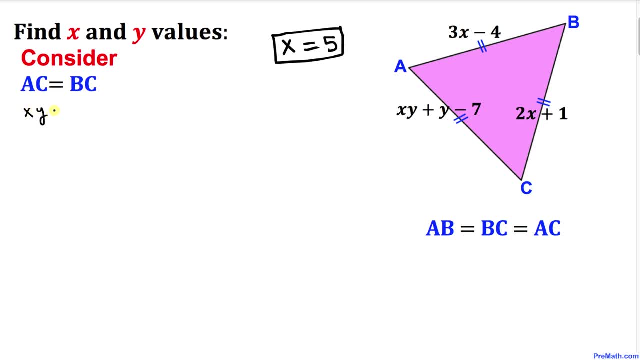 so we can write it as x, y plus y minus 7 equals to 2 x plus 1. all right, now let's go ahead and move this negative 7 on the right hand side. so we got x, y plus y equal to 2 x plus 1, and this negative 7 is going to become positive 7. 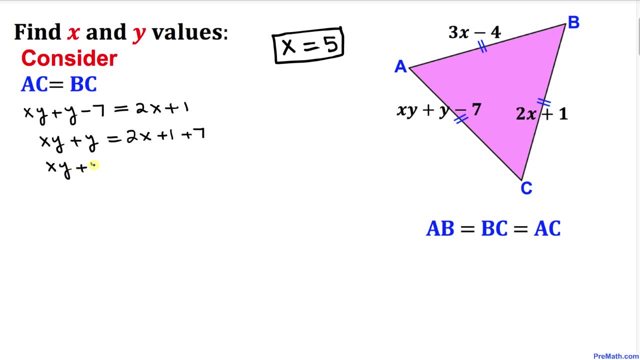 so thus we got x, y plus y equal to 2 x plus 8. and now we are going to substitute x equal to 5 value in this equation. so wherever we see x, i am going to replace that value by 5. so we got this one: 5 y plus y, equal to 2 times 5.